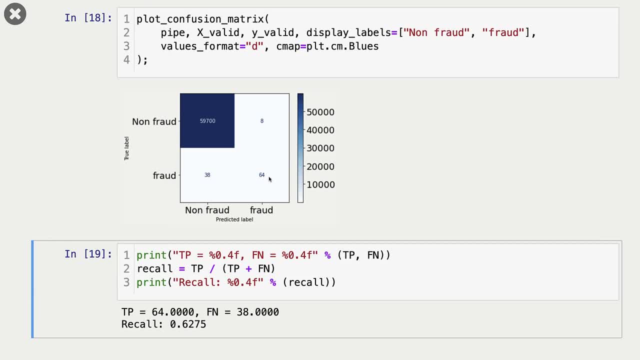 And we have 64 true positives because we are considering fraud as our positive metric And our recall was 38 true positives from our positive class And we have 38 false negatives. So these are the examples that were missed by our logistic regression model. 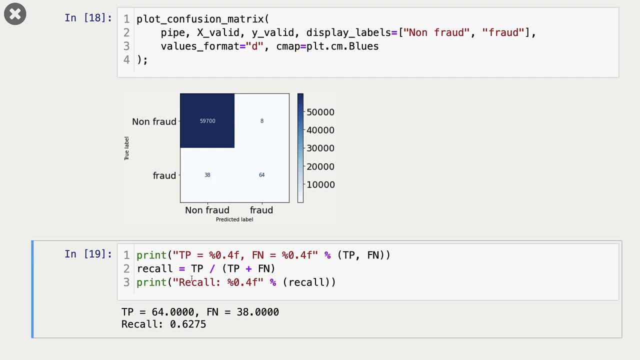 So our recall is going to be 0.62. Okay, So we have 64 true positives and 38 false negatives. Okay, so this is interesting because our accuracy with logistic regression was negative. Okay, So this is interesting because our accuracy with logistic regression was negative. 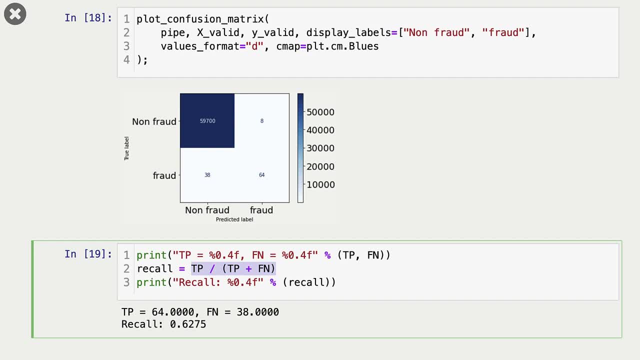 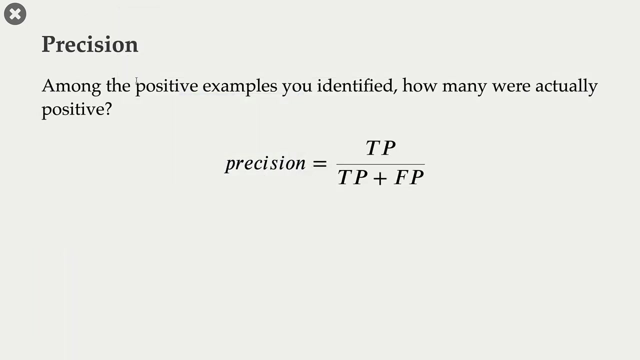 0.9991.. And when you look at this different metric recall, we get this recall of 0.6275.. So the model is not really doing very well here. It is missing many fraud transactions. Our next metric is precision. Precision tells you among the positive examples you identified. 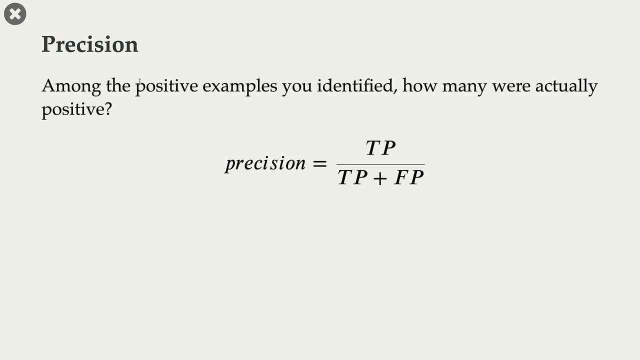 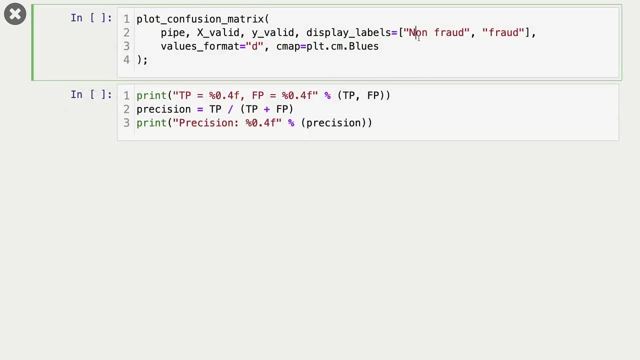 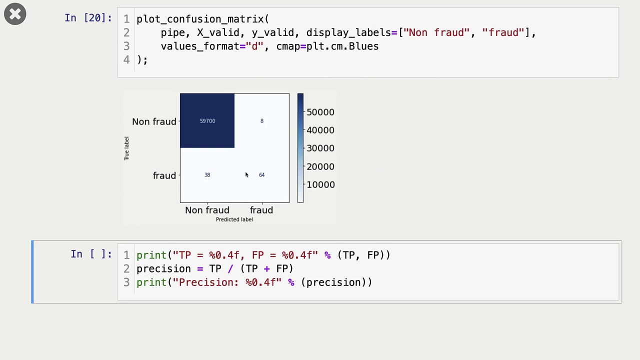 how many were actually positive. So the formula for precision is true positives over true positives plus false positives. And here is our confusion matrix. And how many true positives do we have? We have 64 true positives. So the numerator is the same for recall and precision, but the denominator is different. 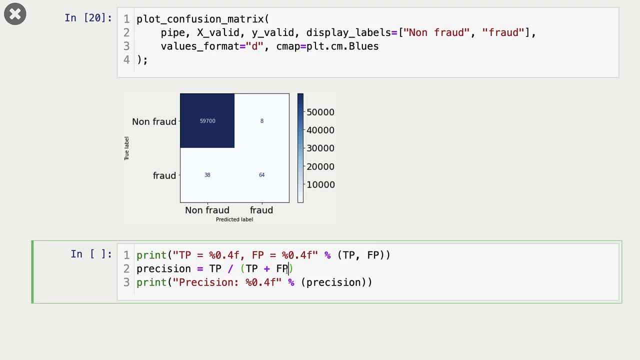 So we have 64 true positives and 8 false positives. So our precision is going to be 64 over 64 plus 8, which is 0.8889.. So logistic regression is giving a reasonable precision score of 0.8889,, but kind. of a low recall score. The reason for that is that the number of false positives is very low. So we have 64 true positives and 8 false positives. So our precision is going to be 64 over 64 plus 8, which is 0.8889.. 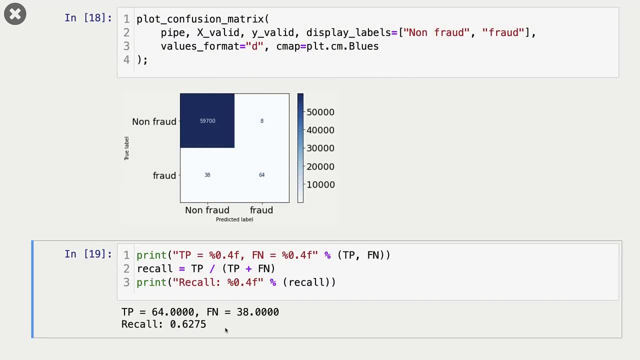 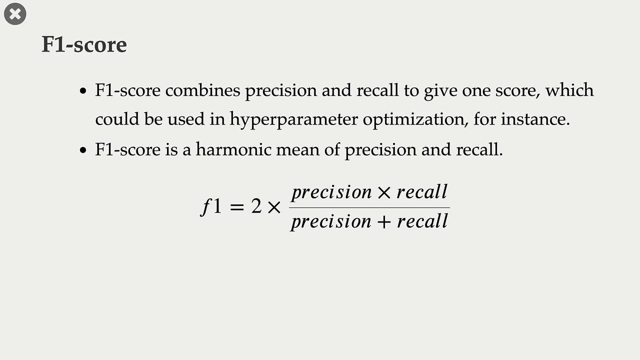 score in this particular case. very often you need one number or one score to use in, say, hyper parameter optimization. f1 score combines precision and recall and gives us this number. it uses this formula to calculate the score and let's calculate it on our own. in our case, 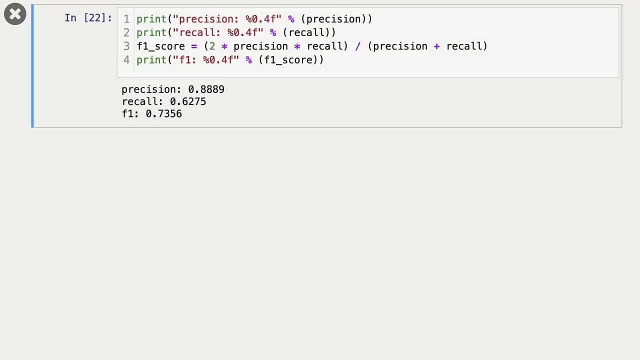 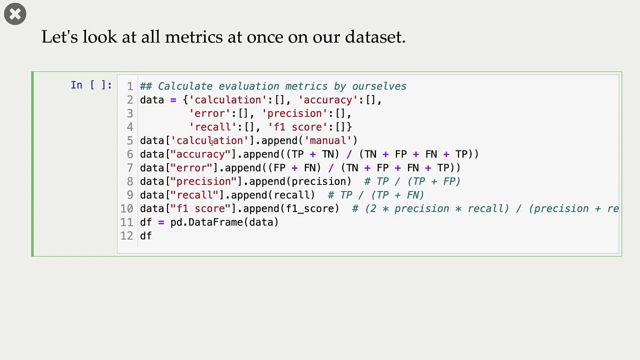 our f1 score is 0.7356. let's look at all metrics at once on our fraud data set. in our case, accuracy is pretty high. 0.999 error is pretty low. precision is reasonable. 0.888 recall is kind of low and f1 score is also kind of low. 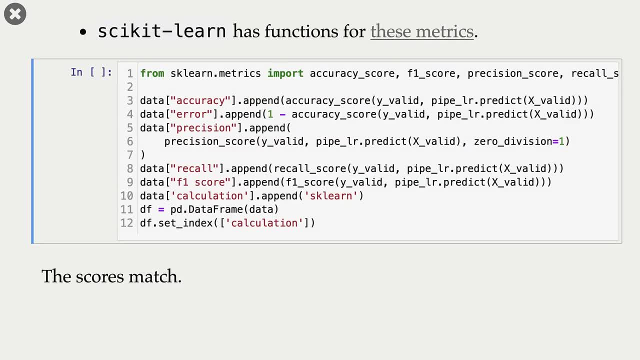 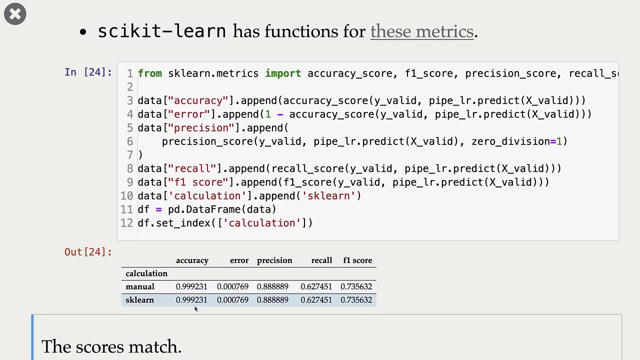 in the previous slides we calculated precision, recall and f1 score on our own. now scikit-learn also has functions to calculate these metrics and you can import them from sklearnmatrix. and here i'm calculating all these metrics. as we can see here the scores calculated by us and scores given by scikit-learn- they match. so this is. 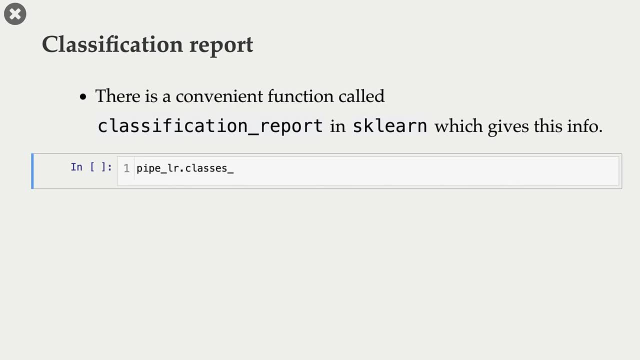 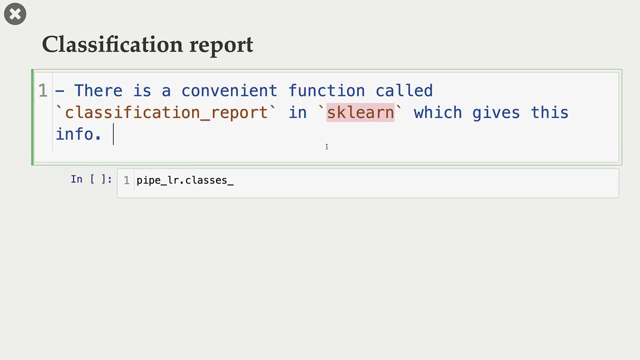 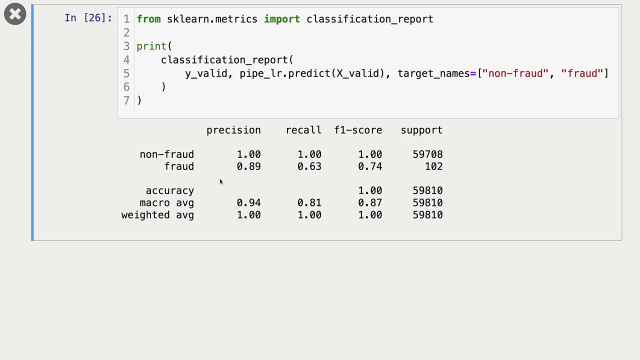 good. scikit-learn provides this convenient function called classification report, which gives us all information about precision, recall and f1 score. so these are our classes: zero and one. i'm giving them names. uh, for zero i'm calling it non-fraud and for one i'm calling it fraud. 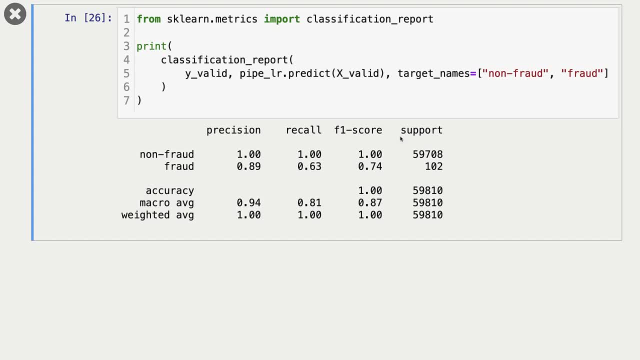 there is precision, recall and f1 score for fraud as well as non-fraud. so before we were considering fraud as positive class. but in this classification report it considers each class as positive and calculates precision, recall and f1 score. so these scores they match with what we got before. 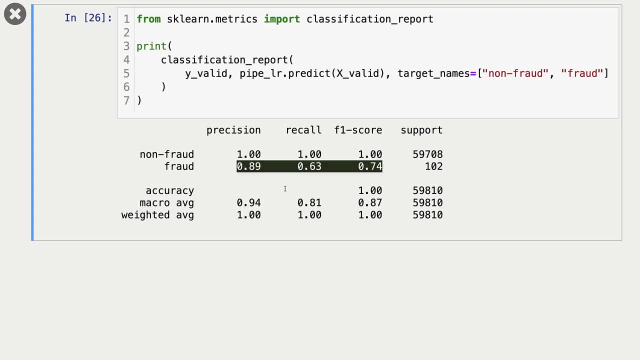 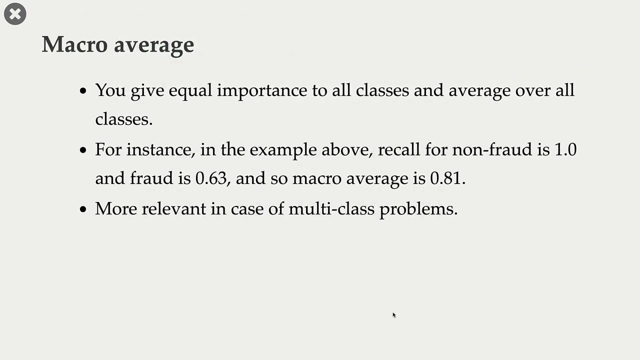 when we consider fraud as positive class and these scores non-fraud. we didn't calculate, but these are calculated by considering non-fraud as the positive class. we also see macro average and weighted average here. what do they represent? macro average gives equal weight to different classes. in in our particular case we uh. fraud class was more. 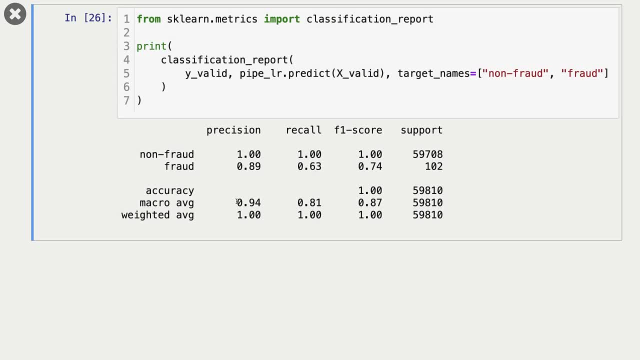 important to us, and so we only looked at precision recall and f1 score for fraud class. but in some cases both classes are important, or if you have multi-class classification problem, then you have different number of examples for each class, but precision recall and f1 score for all classes. 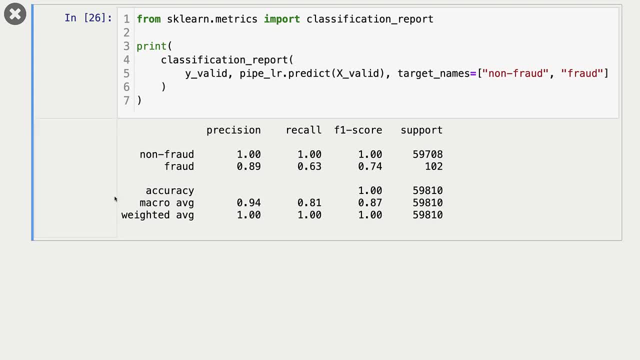 is important to you. in that case, you would go with macro average. you want to give equal importance to all classes. on the other hand, in case of weighted average, you give equal importance to each example. so in our particular case, non-fraud has more examples and so weighted average is one here. 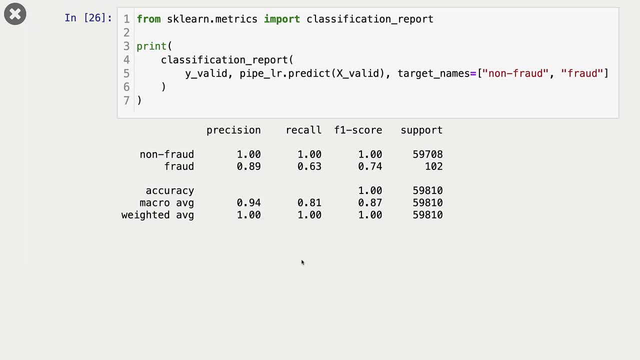 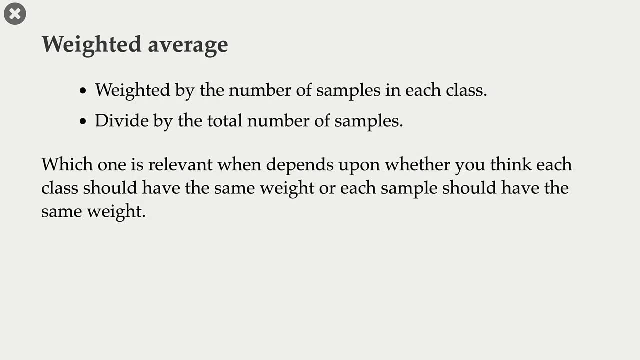 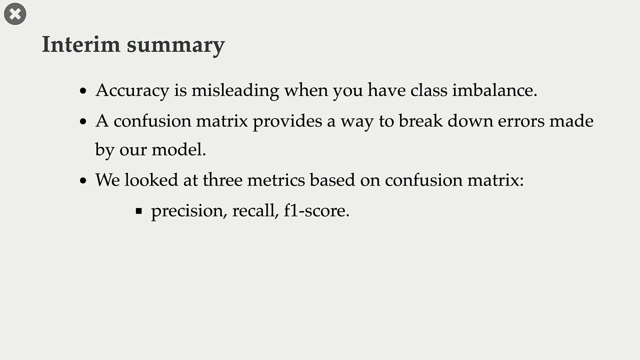 now, which one should be used in what context is up to you. if, in your problem, all classes are equally important, then go with macro average, and if each sample is equally important, then go with weighted average. okay, so far. what all things have we seen? we have seen that accuracy is misleading when you have 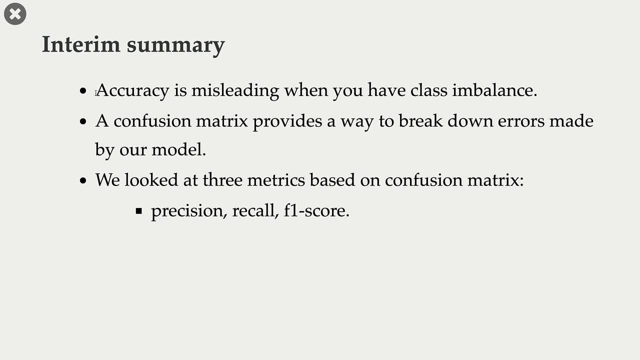 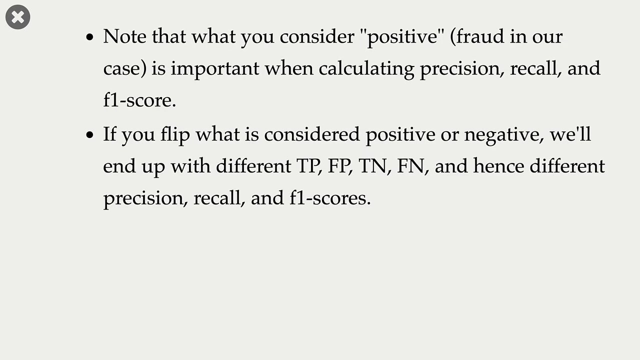 class, imbalance. confusion matrix provides this nice way to break down errors made by your model. we looked at three matrix which are based on confusion matrix, precision recall and f1 score, and it is important what you consider to be the most important in your model as positive class when you are calculating precision recall and f1 score. if you flip, 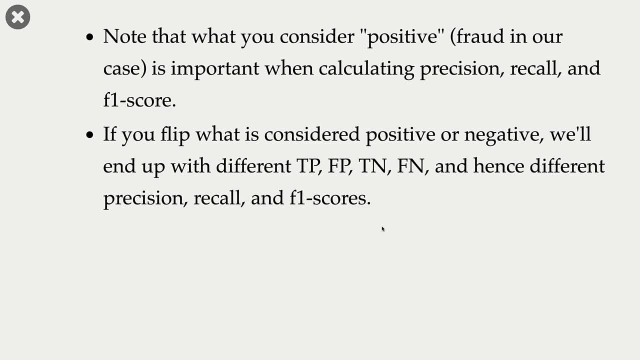 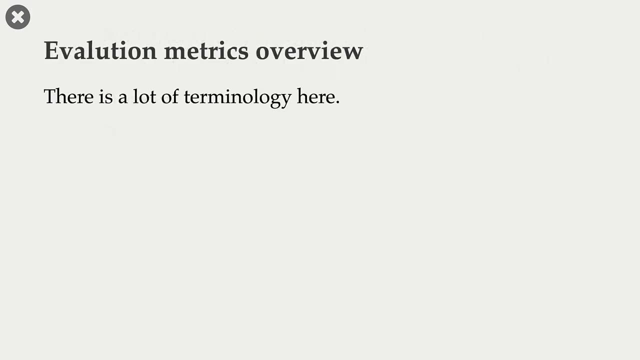 what is considered as positive or negative. you are going to end up with different true positives, false positives, true negatives and false negatives, and so you will have different precision, recall and f1 scores. now, in this lecture so far, we have looked at many definitions and there is a lot. 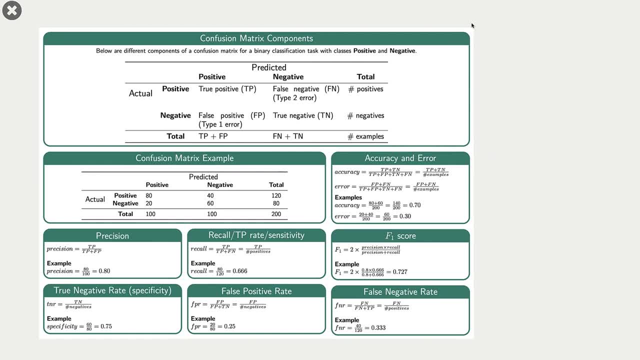 of knowledge here. i have created this cheat sheet which has definition for confusion, matrix and accuracy, precision, recall, f1 score. there are also these other terms. people tend to use true negative rate, false positive rate and false negative rate, so you'll find all the definitions and examples for each in this cheat sheet.